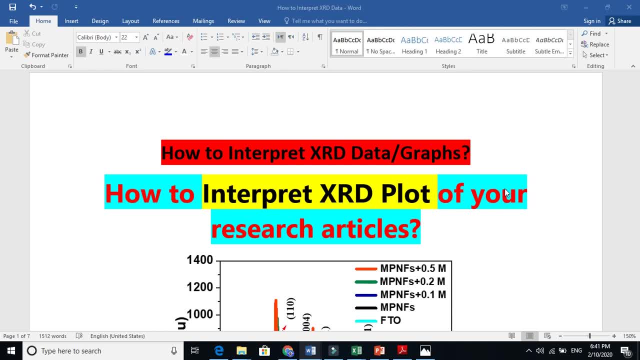 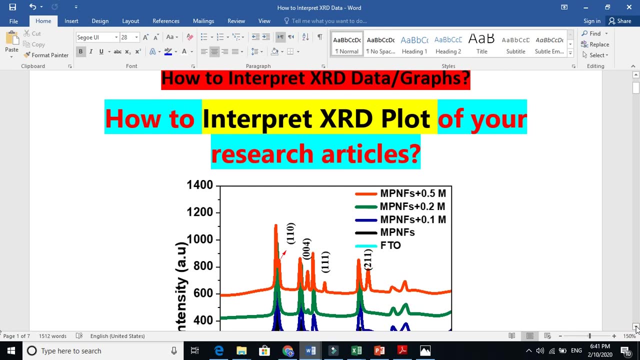 In this video I'm going to talk about how to interpret XRD data or graph of your research article. When you are writing your research article- how to interpret XRD plot- It is one of the key characterization in your research and you need to write about in your 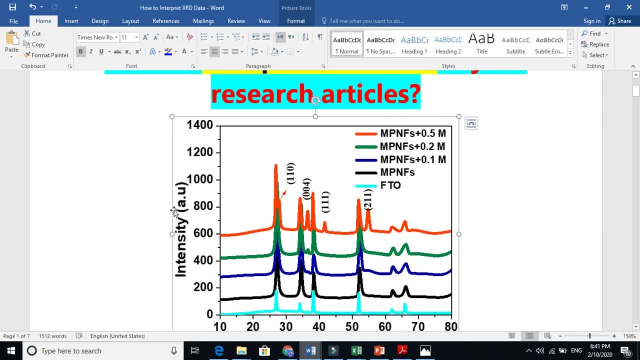 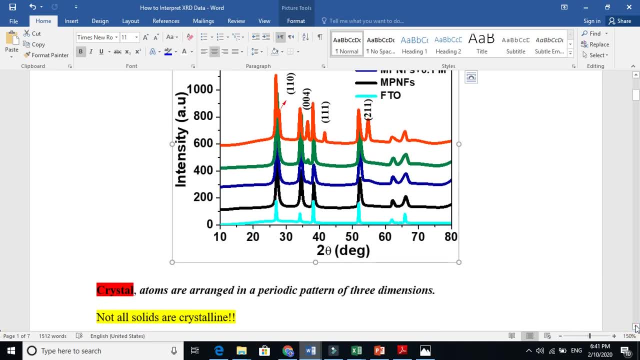 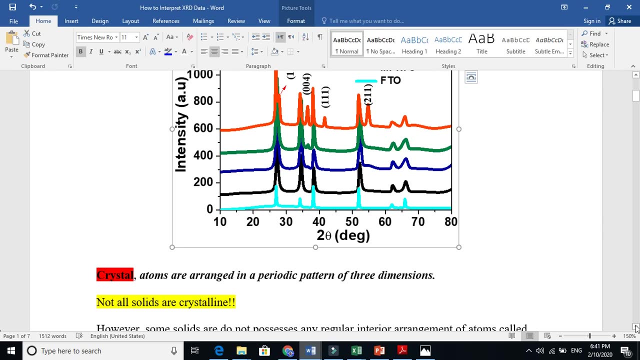 research article. This is, for example, the graph we plot: intensity versus 2 theta. Let's give me first of all a brief introduction that why we need to do these characterizations. For example, you are working in a material and you want to know that either. 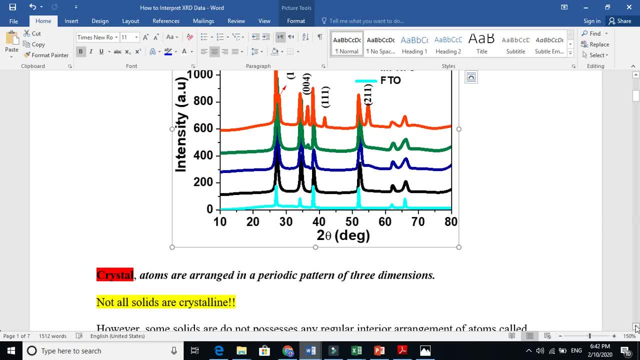 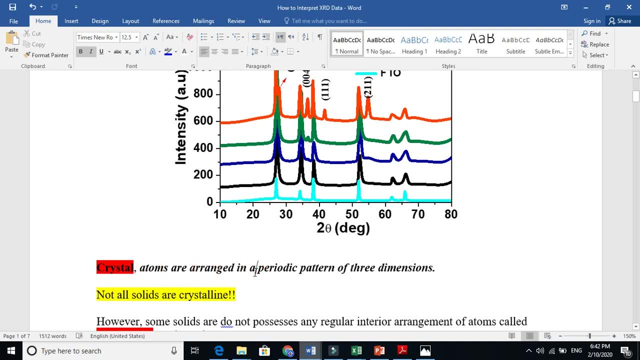 this material is a crystalline or a marpous, For example. if it is a crystalline, so crystal means that atoms, those atoms are arranged in a periodic order. so it will give us a certain crystalline or a marpous, So crystalline means that atoms are arranged in a periodic order. 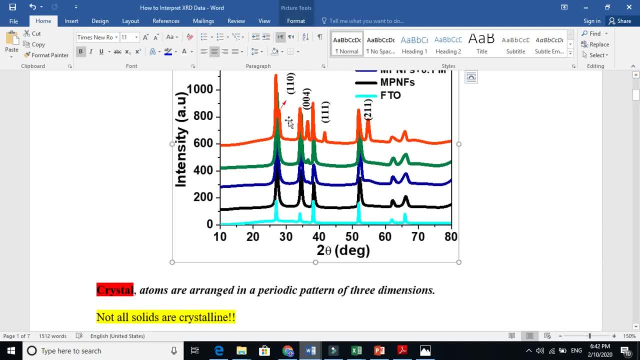 So crystalline means that atoms, those atoms are arranged in a periodic order, So it will give us different peak. for example, if a material is a crystalline, so it will give a sharp peak. so you can easily understand when i see the xrd graph, so i can see that this is crystalline or amorphous. 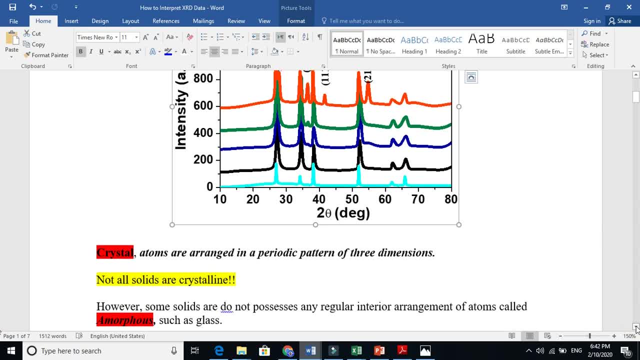 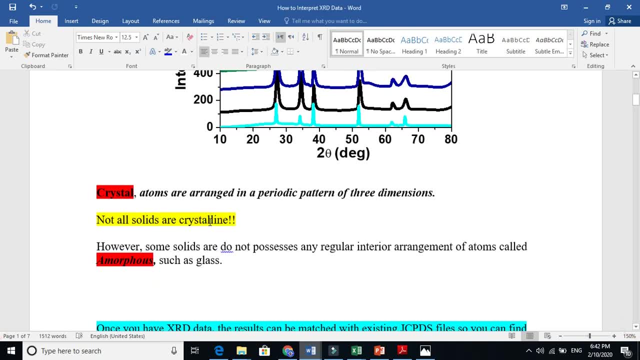 i will explain in the next video what are the differences between amorphous plot and in crystalline plot. now, all solids are not crystalline, some are positions, irregular order of the interior atoms and that we call amorphous. here you see now, once you get your xrd data for 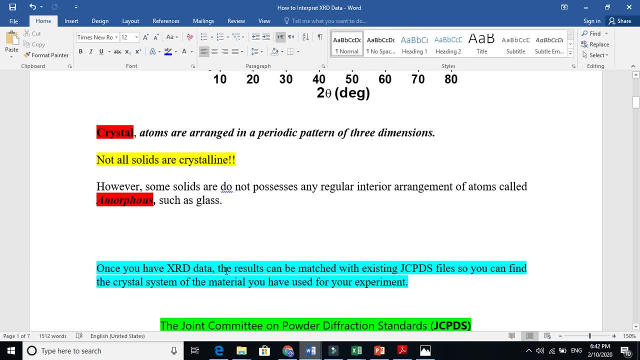 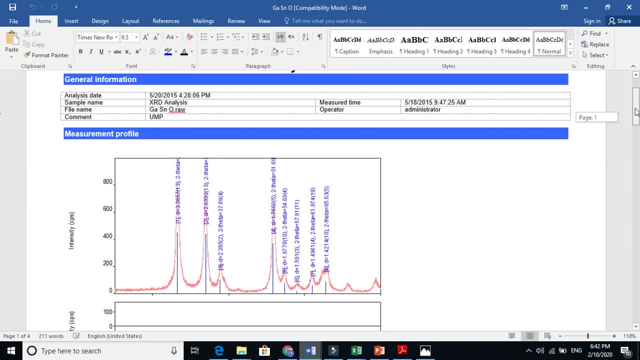 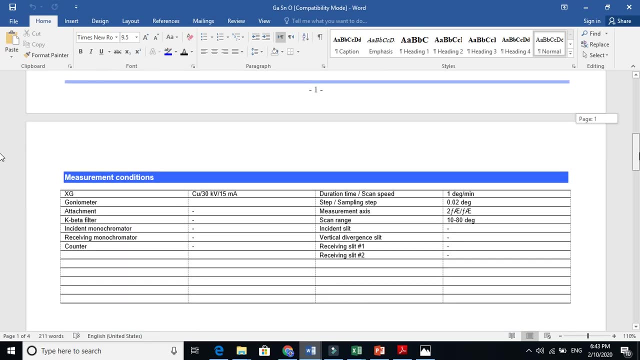 example, when you give your material to the xrd machine. so they will give you two file one. they will give you this file in ms world so you can see the material name, uh, the place name, and this is the graph you see here. you can see all the information here and this is another graph. 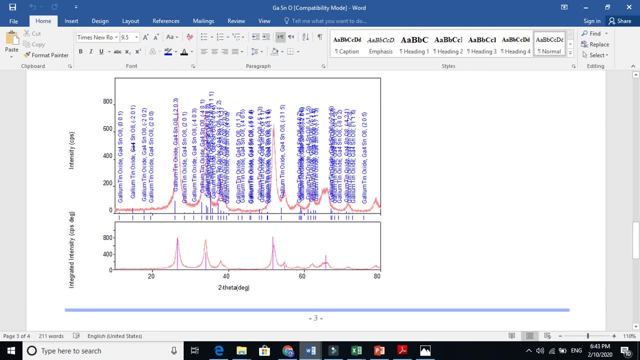 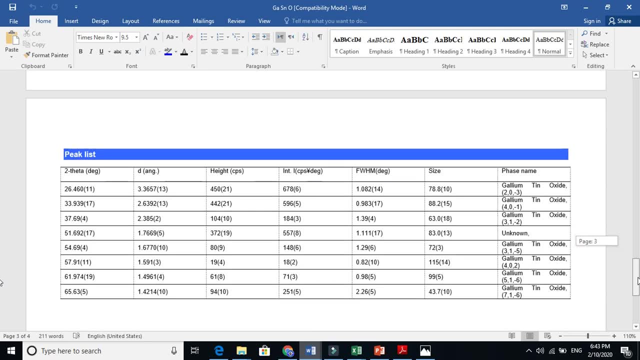 they have and the peaks are automatically indexed- that this two one zero one peaks are lying in this two theta and etc. let me explain to you here, and it will also give you the graph here, the the table here: uh, in this two theta, two theta angle, the despacing is this much and the pull width, hop maxima is this: 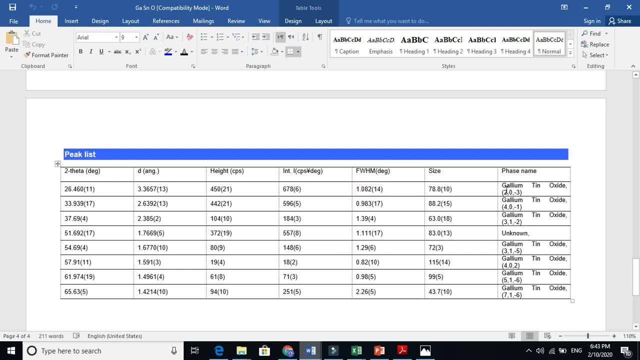 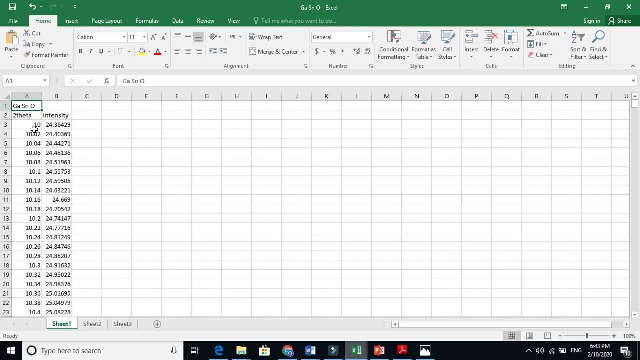 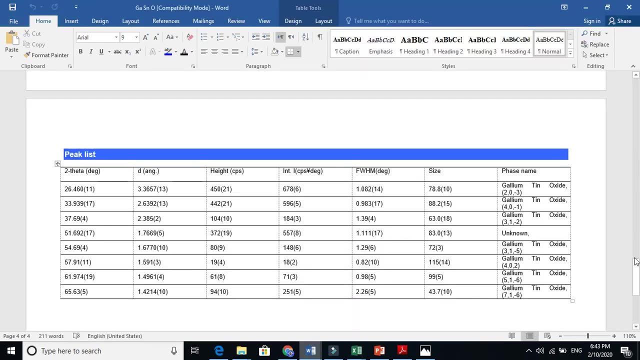 much and the, the, the, the peaks, uh, the plane, the hkl value are here and it will also give us the second file and that is in excel. this is the two theta and this is the intensity. so, if you do not like these graphs, in in ms1 the ready-made graphs, these graphs, so you can use this excel data. 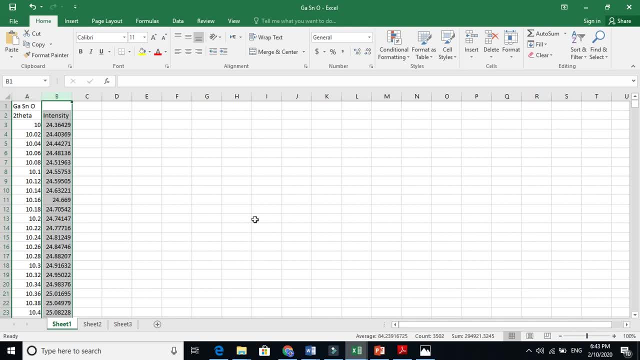 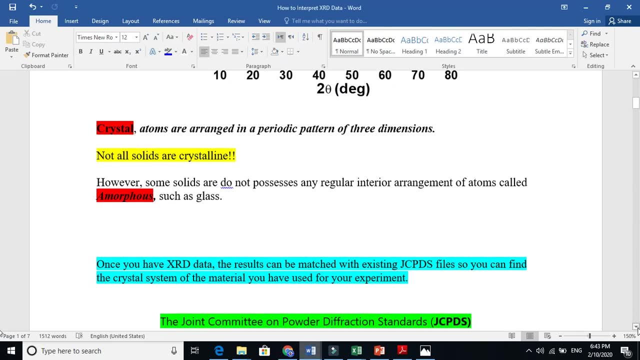 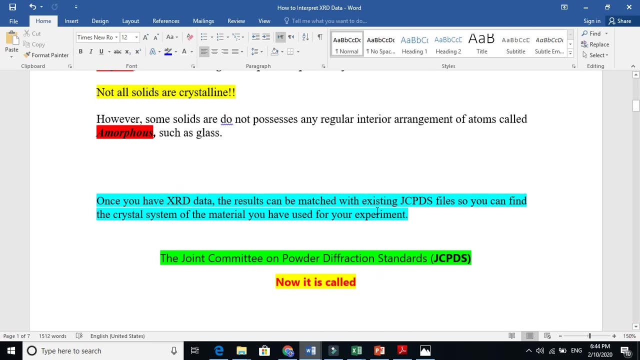 to plot by yourself in the origin. okay, now let's go and see how we index these xrd data. so once you get the xrd data, the results we match with the existing g, c, j, c, p, d s file. this is all periodic table elements. they have a proper number and they given the proper number. this means the joint committee. 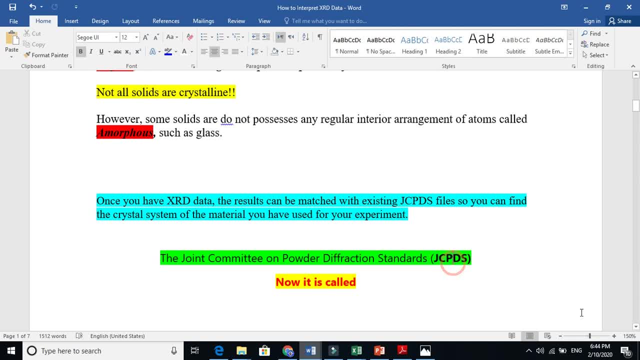 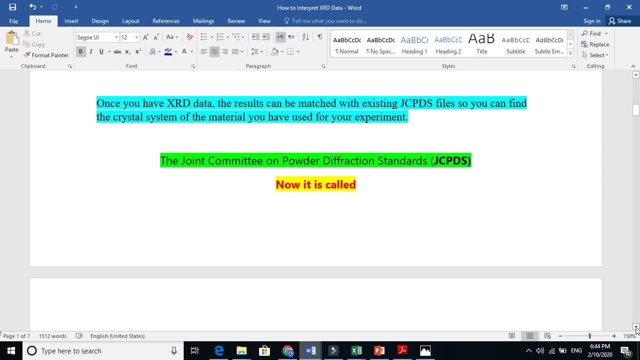 and powder depression. standard g, j, c, p d s. we compare our peaks, our two theta d value, with the standard value if it is matching. for example, i am working in pure tenax side when i compare my xrd data with the standard, with the standard j c, p d s value if it is matching. 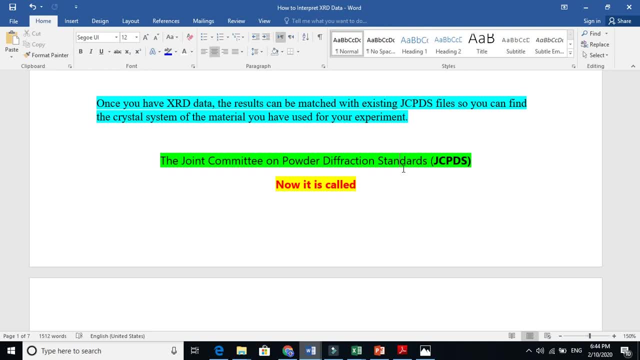 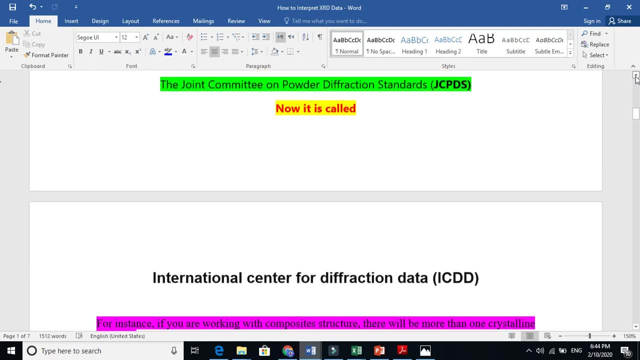 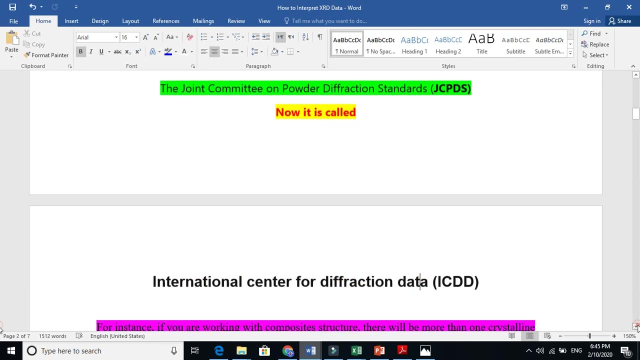 then i am pretty sure that i synthesize my desire material. look now, and this j, this j s, this j c p d s is nowadays called international center for depression data, icdd, so currently it is called like this. let me give you a little bit of an example of the xrd data. so let me give you a little bit. 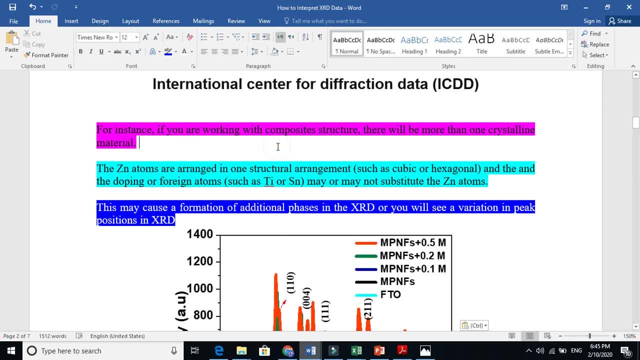 of a brief overview here. for example, if you are working with composite material, right, and you say that there will be more than one crystalline material, for example, your host atom is zinc and you know zinc has a proper arrangement, such as cubic or hexagonal. okay, such as cubic or 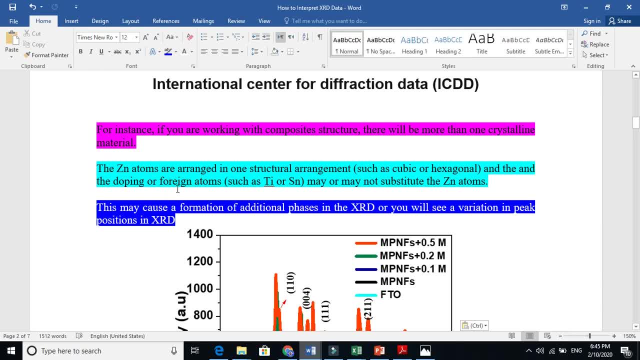 hexagonal and you want to do off or bring some foreign atom, make a composite of titanium and ac. so it may or may not be a composite of titanium in acid. so it may or may not be a composite of substitute. the zinc atoms, for example, if the zinc atom and titania are sn, have the same atomic size. 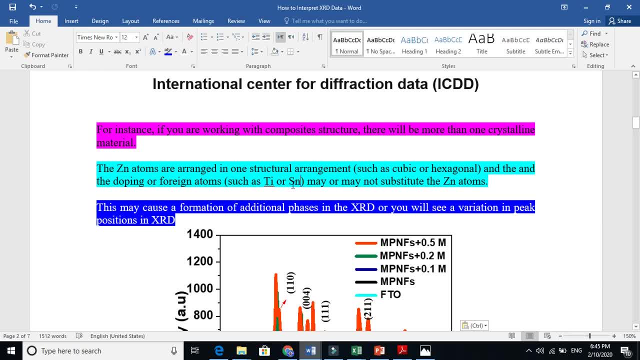 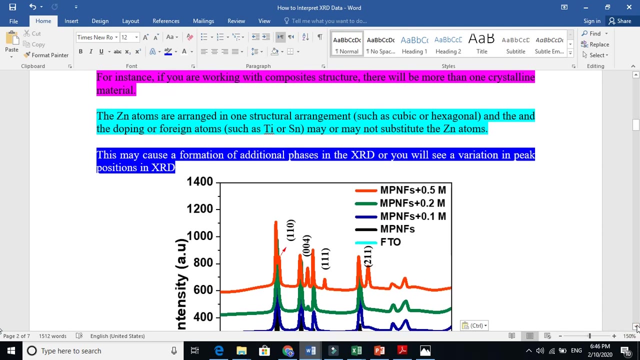 so it will cause no problem. but if it is not substitute, so it will make interstitial doping and it will deform the host atoms, so the host material, so it may cause in additional p pages in xrd, or you will see variation in the peak position of xrd. so from this kind of thing 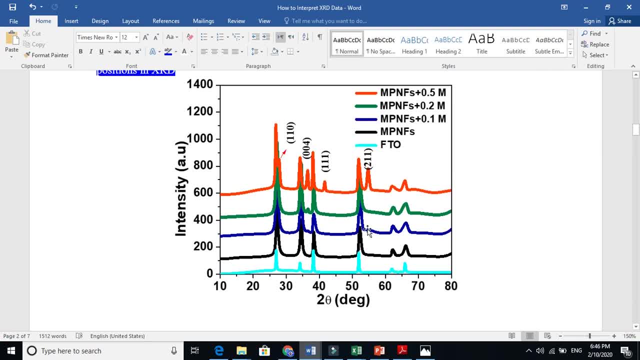 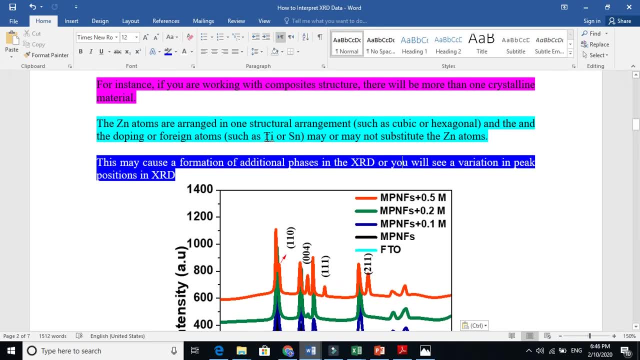 you can easily understand it, whether my peaks are disturbed or not. for example, i told that every material healthier standard uh, will you up d and planes or everything? now, if you are doing doping, are you making composite and you know the pure zinc oxide or zinc xrd data and when you incorporate these atoms? 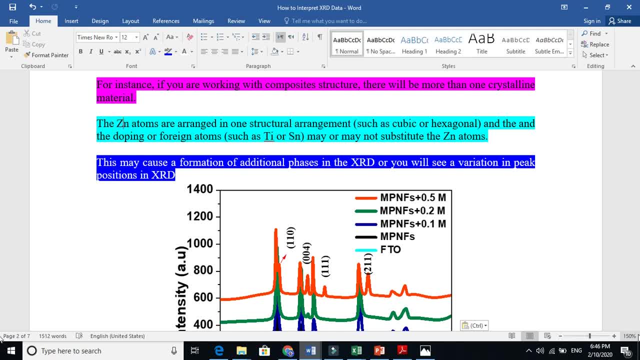 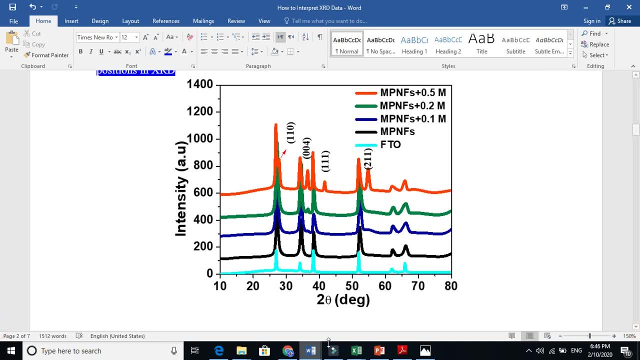 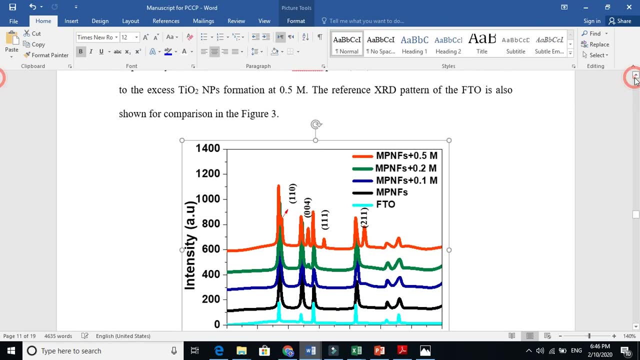 in the zinc and you see some variation and some other peaks, so you can clearly say that a composite is farmed very, very clear. so let's go now to the real scenario and, uh, how i write my xrd data here in my paper. okay, look now the phase. 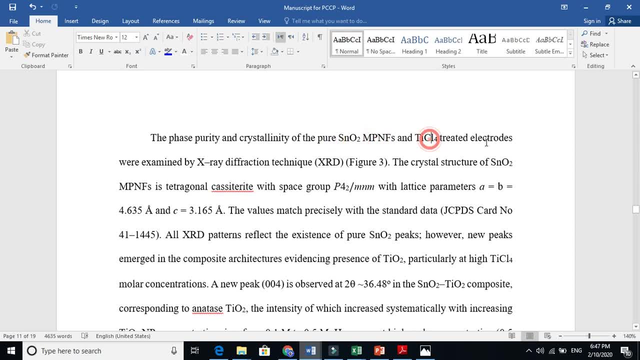 i will be looking at the xrd taken on the xrd data and then the amount of the xrd that we get when we are taking xrd data to this xrd machine, and then what the xrd data in here. what is the xrd data which is necessary to work with the xrd data? so let's see, say that the xrd data is: 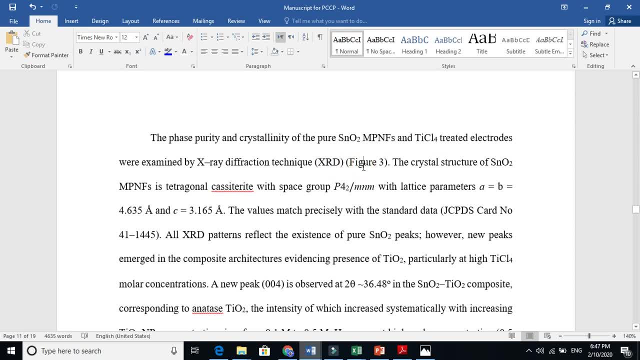 xrd and we are measuring the xrd and the concentration a. i will use xrd as the zc here. so the x dr, initial xr t will be the value of max to t. so its real value in terms of its form- and this is the xr d and t- is equal to the xrt of the p1c2, and so my xrd data is the ordinary. 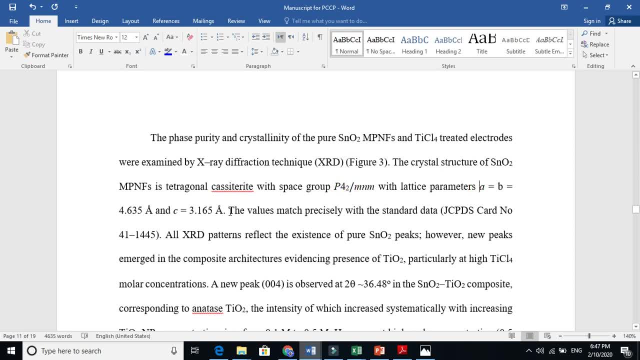 where the latest parameters are this and this. the values met precisely with the standard data: J, C, P, D, S, Cod number. I told you, remember, I told that all these things have their value. All XRD patterns reflect the existence of pure SN2 peaks. 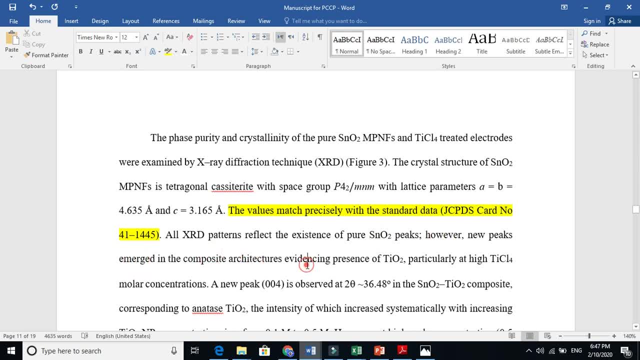 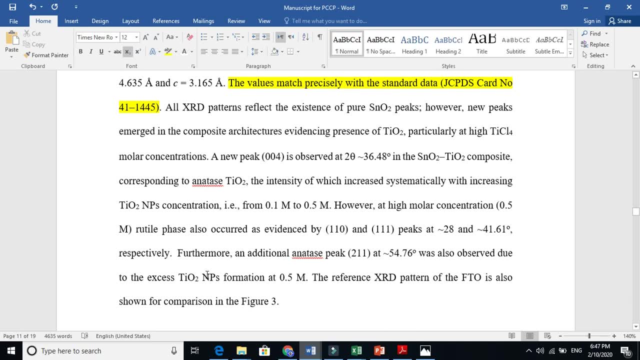 However, new peaks emerge in the composite architecture, evidencing presence of titania. I told you before you see, So this is how you write, And you just write all about this. And I also mentioned here that there are some rotile phases occur because of the titania composite.